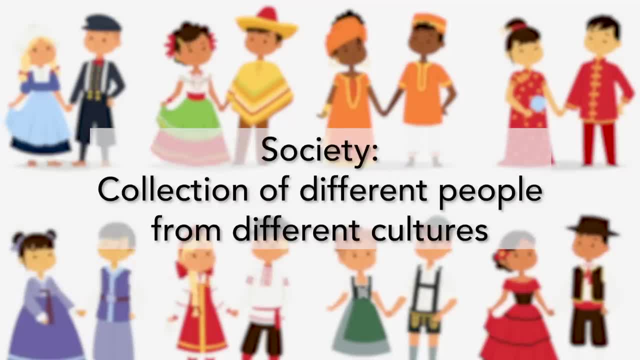 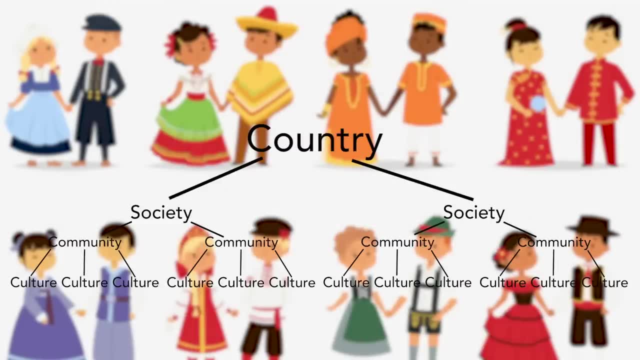 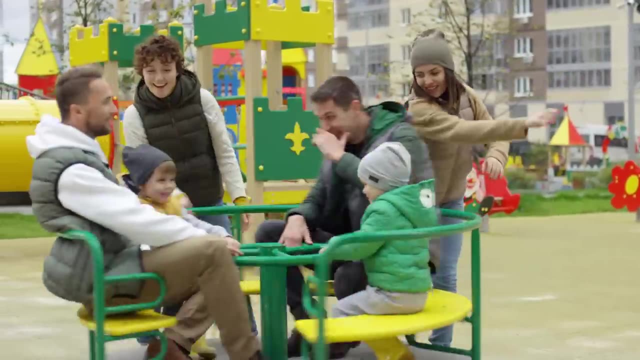 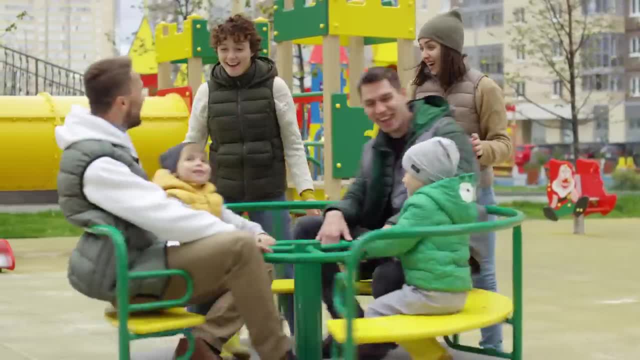 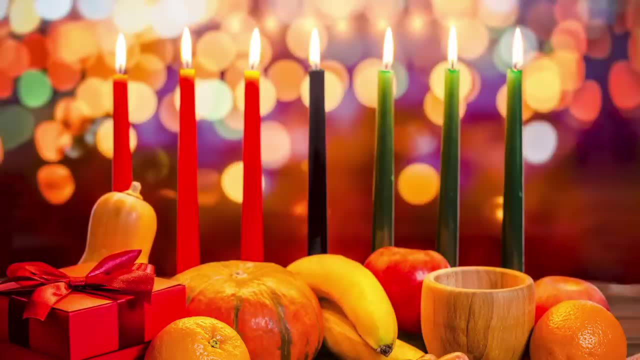 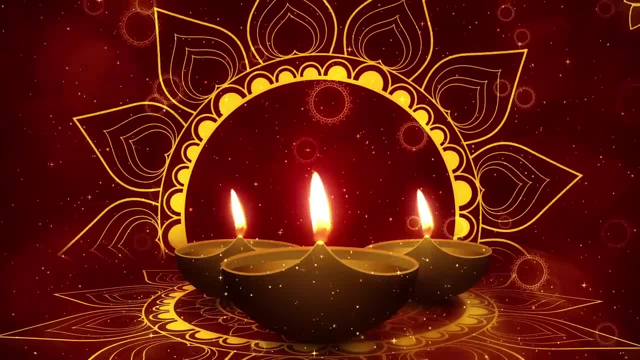 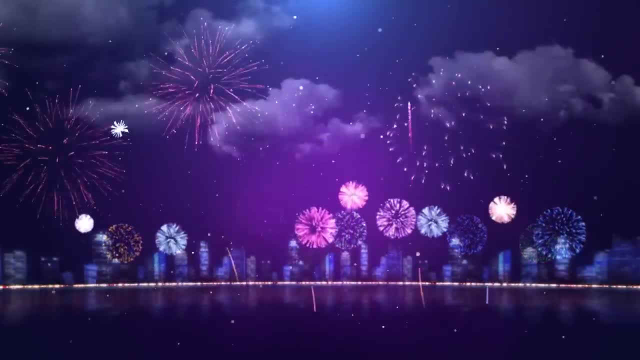 St Nicholas Day or St Lucia Day Again, others might celebrate holidays you've never even heard of, or none at all. All year round, there are holidays, parades, shows and events that different cultures celebrate or attend that others do not. Every culture. 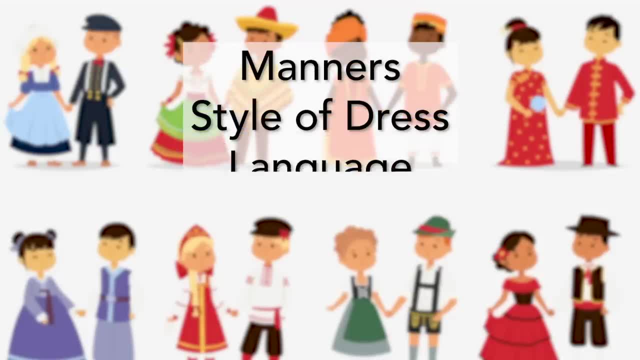 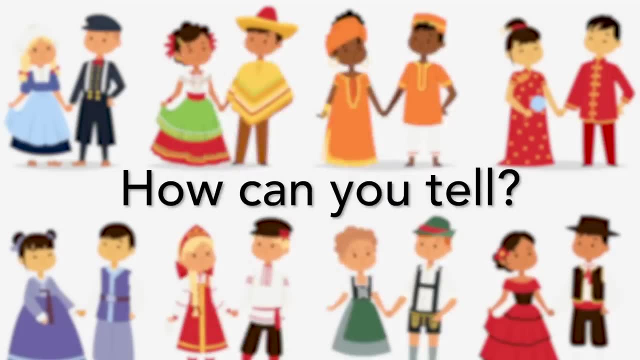 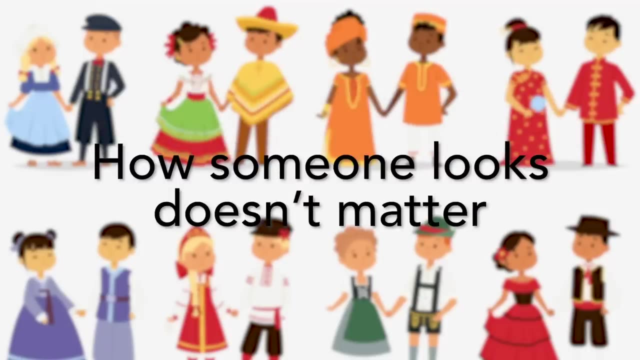 has its own unique manners, styles of dress, language, religions, celebrations, ethics and other things that are special to them. So how can you tell what culture someone belongs to? Well, it's important to remember that- the color of their skin or the way they look. 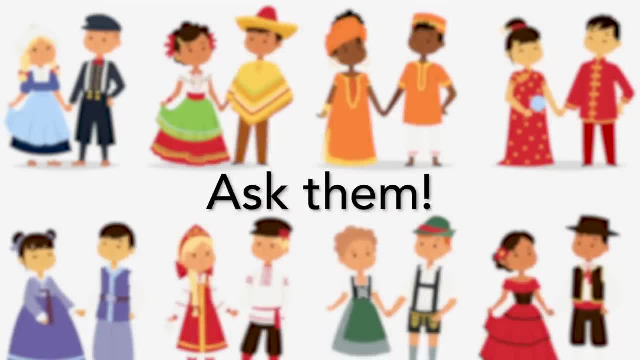 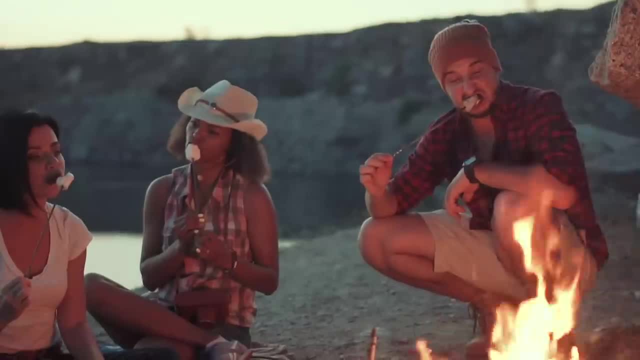 does not define their culture. The best way to find out what culture someone belongs to is simply to ask them. Have a conversation, Find out more about them. Maybe you have some things in common. Perhaps their culture and yours have some of the same likes and dislikes. 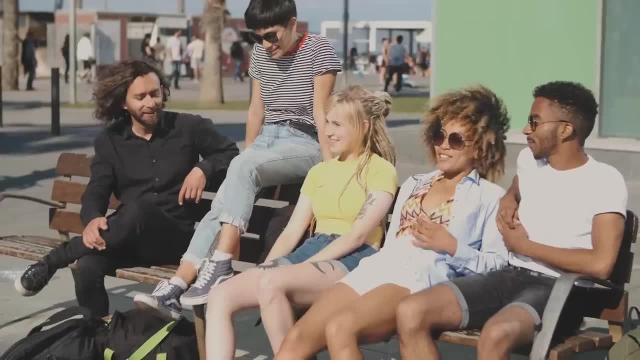 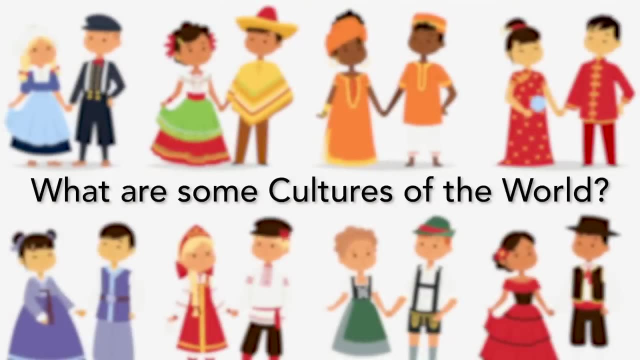 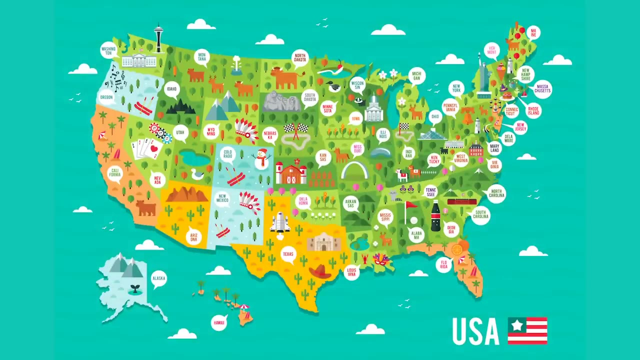 or hobbies or foods? Maybe not. Either way, it's good to share these things so you can learn more about the people around you. So what are some of the cultures of the world like? Let's start with America. Some of the foods that are part of the American culture include pie. 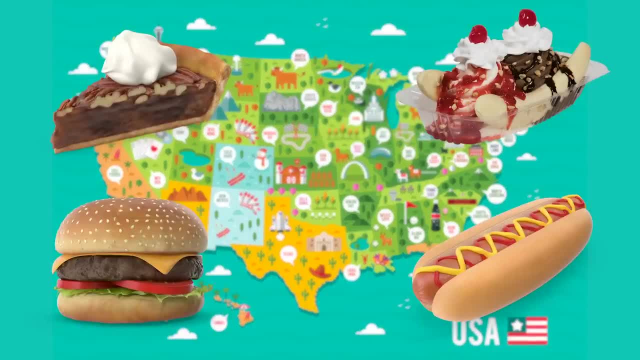 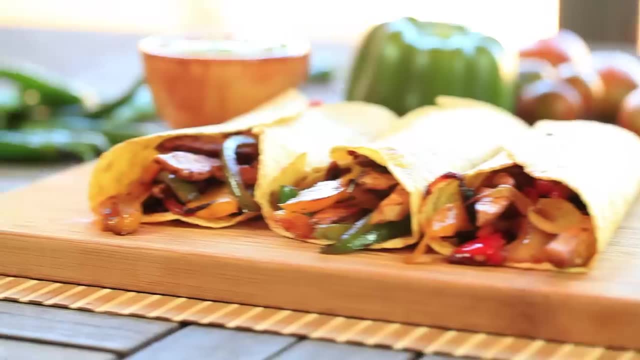 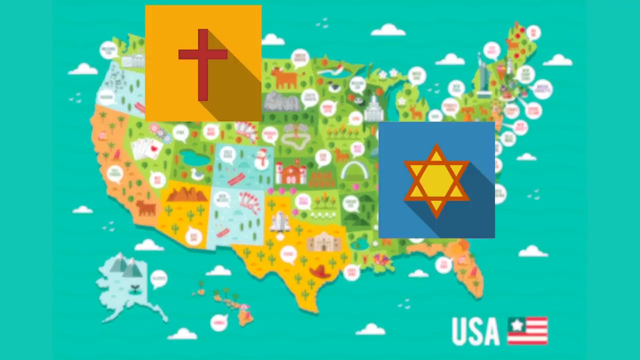 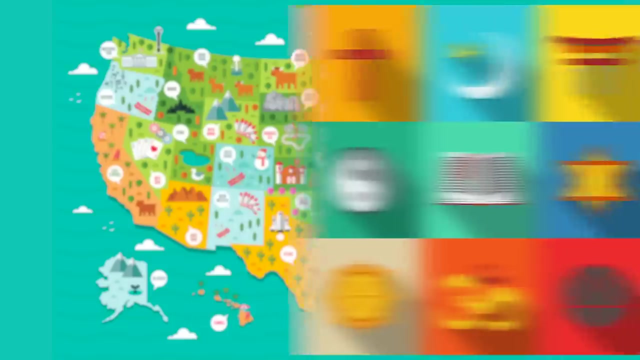 banana splits, hamburgers, hot dogs and fried chicken. Other American populations have different preferences. For example, in the Southwest there is a mixture of Spanish and Mexican foods. Religions in American culture include Christianity, Judaism, Islam, Buddhism, Hinduism and others. Americans celebrate Christmas Thanksgiving. 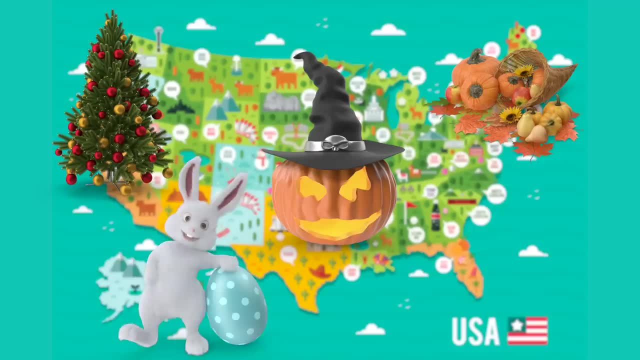 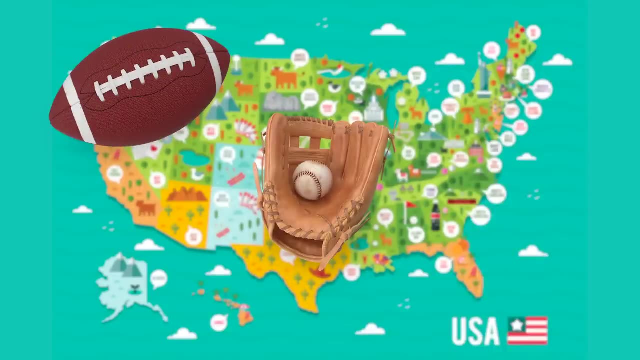 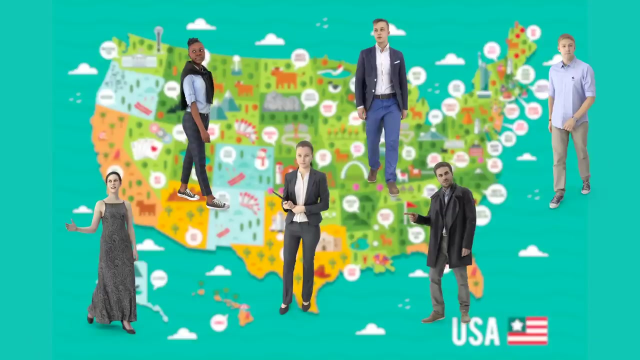 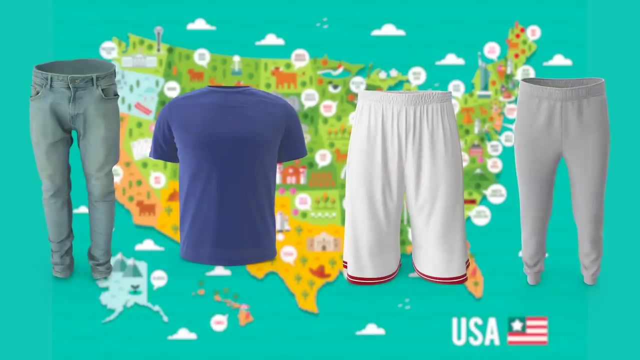 Halloween, Easter, St Patrick's Day and others. American sports include football, baseball, basketball, soccer and hockey. We have lots of different ways of dressing, but American culture is most known for our jeans, t-shirts, shorts and sweats. All of those things help define American culture. 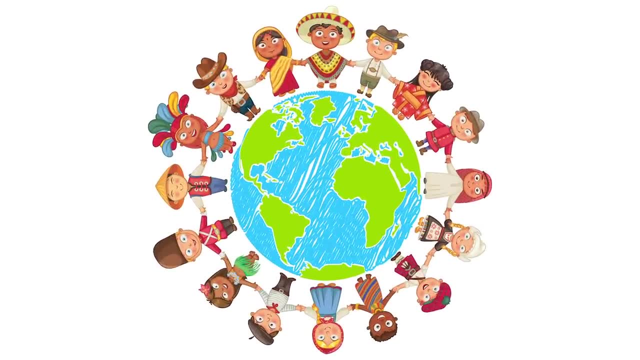 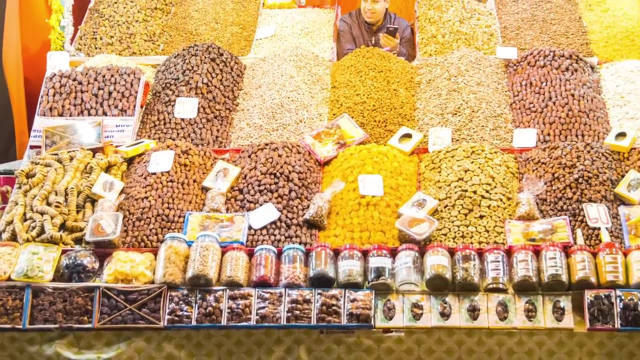 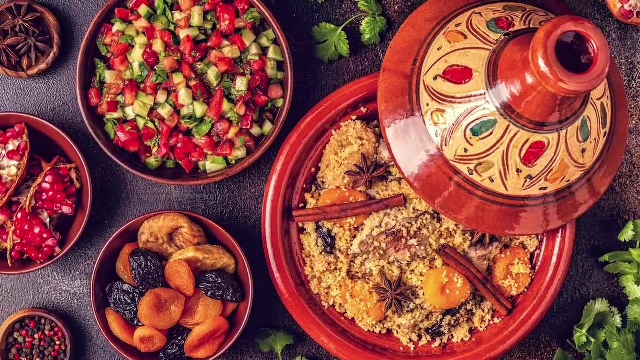 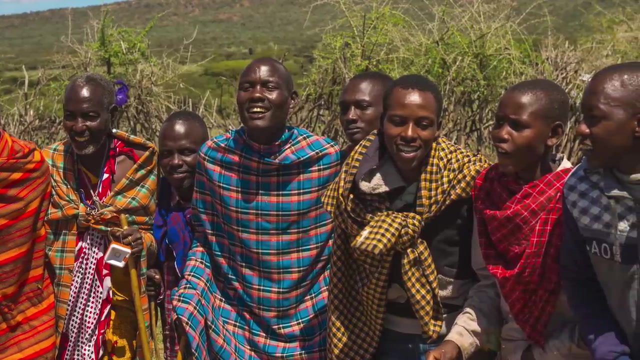 Here are some other cultures and things that help define them. This is Africa. The food across Africa is usually spicy and has intense flavors, and the food can be very exotic as well. They eat many different things that Americans don't. Religions in Africa include Christianity and Islam, but many of the people in more remote parts of Africa practice their own local religions. 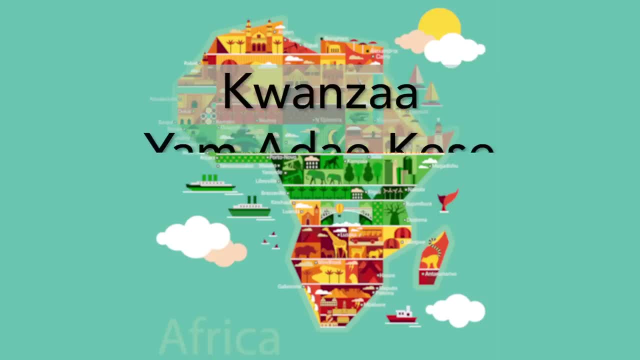 Celebrations include Kwanzaa, Yama de Kese, Zed and Osiris. There's music like samba and reggae. Believe it or not, there are so many local religious. There's music like samba and reggae. Believe it or not, there are so many local religious. 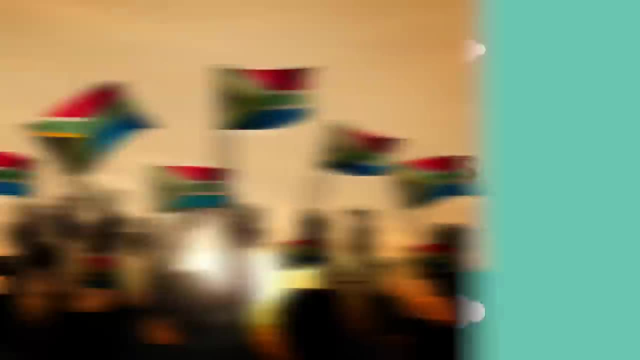 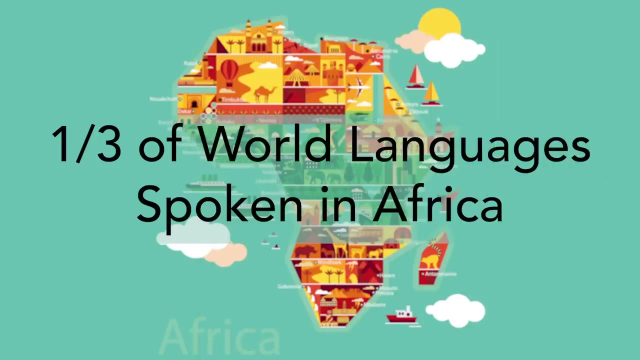 There's music like samba and reggae. Believe it or not, there are so many local religious. There are 11 official languages in South Africa, which is a real rainbow nation where many cultures all coexist. In fact, one-third of the world's languages are spoken in Africa. 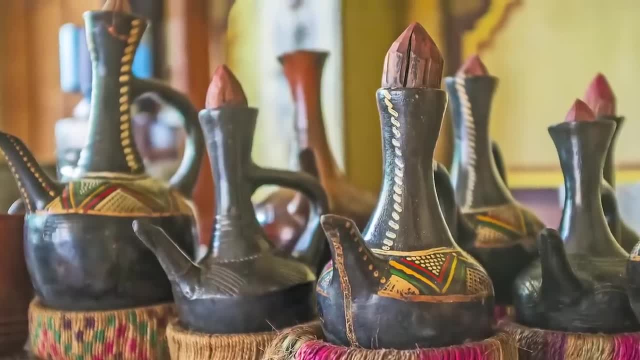 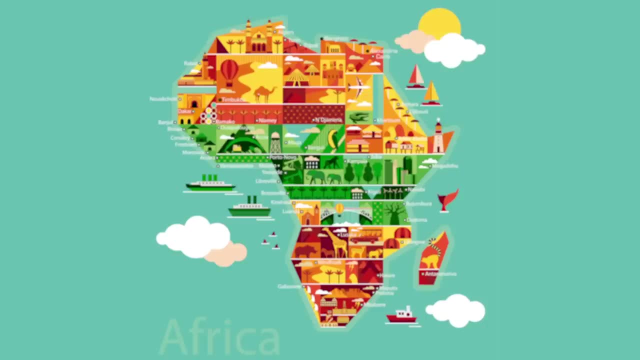 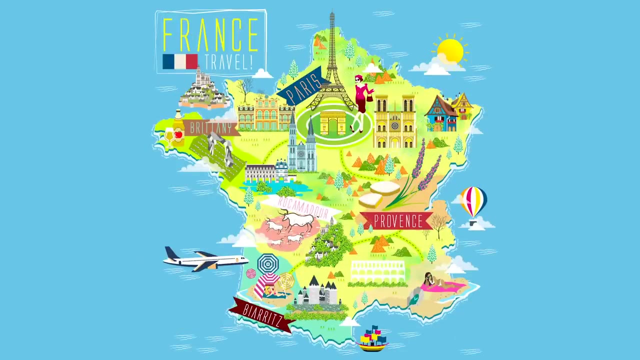 Their art consists of colorful paintings and beautiful ceramics, And the main themes are marriage, mother and child. Unlike American culture, 41% of children aged 5 to 14 work in Africa. What about the French culture? Maybe you know someone French? 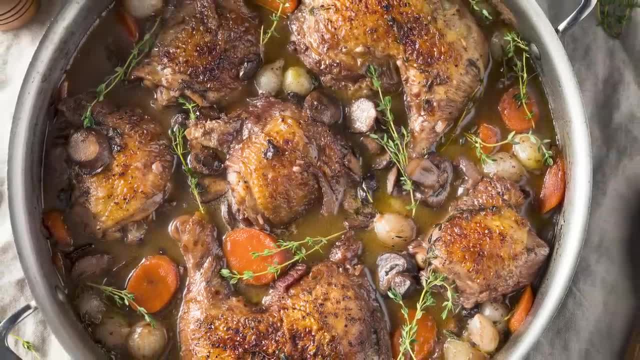 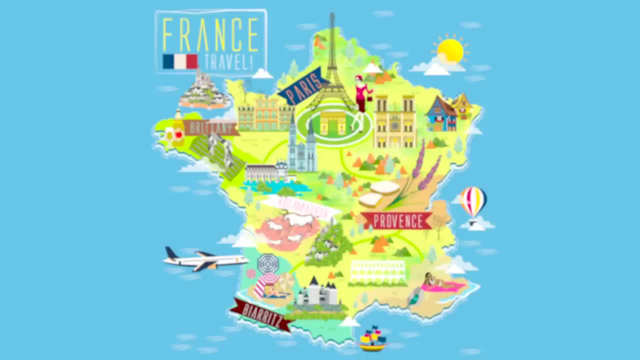 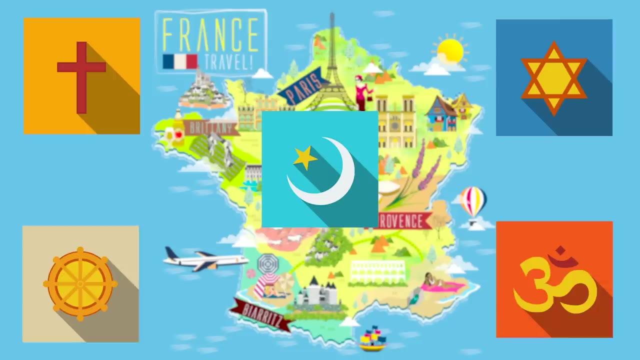 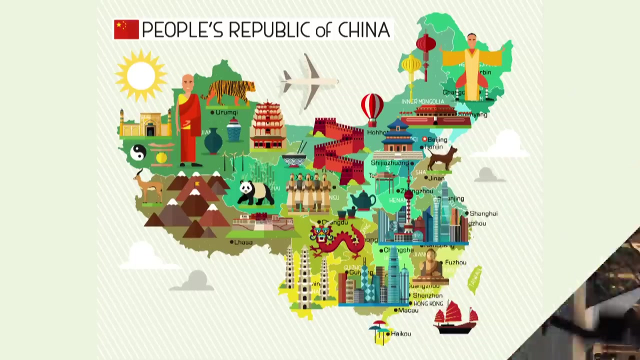 Some of the elements of their culture include complex foods with heavy sauces, elegant and professional clothing like scarves and long coats and dresses. In French culture, religions include Christianity, Islam, Judaism, Buddhism and Hindu. Art and history can be seen in many churches and public buildings. 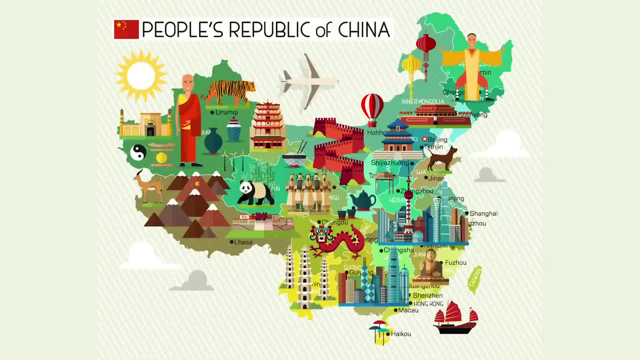 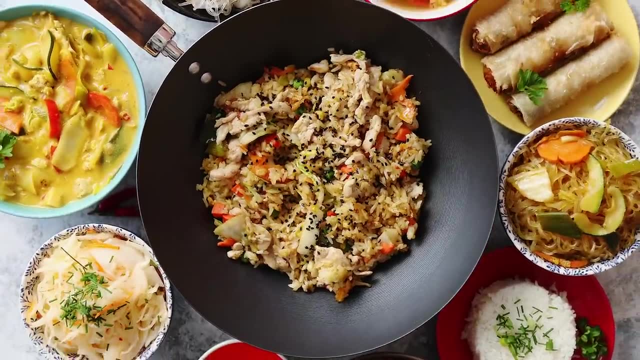 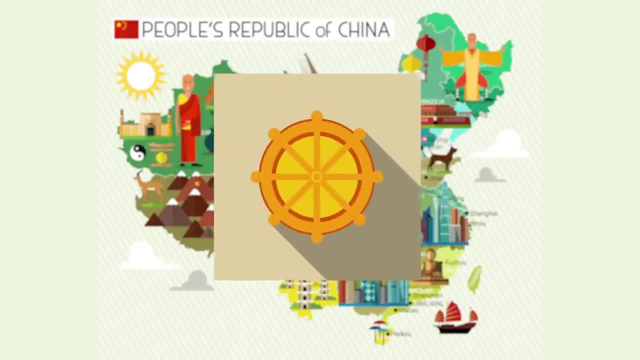 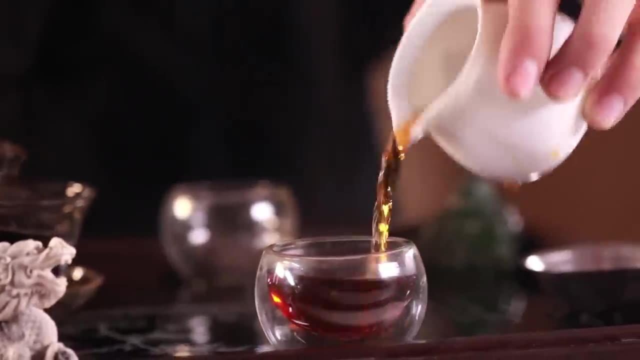 and snakes. The established religion of Chinese culture is Buddhism and there is a lot of Buddhist art there. They drink a lot of tea, which is often used as medicine. The Chinese New Year happens every spring and is marked by a bright and colorful day. 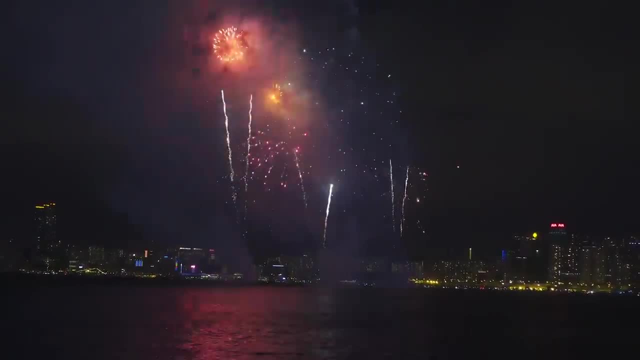 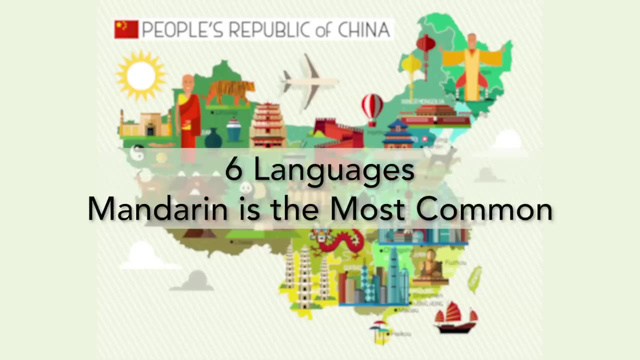 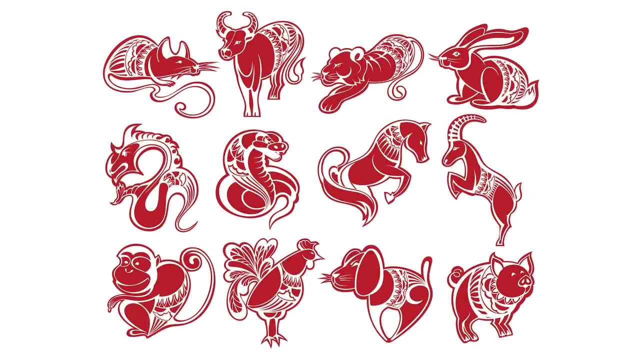 The Chinese New Year is celebrated on the day of the Chinese New Year, so it is often celebrated as a holiday, or Fridays Year in Chinese culture is said to be the most colorful festival of the 15-day day, with a dancing dragon and fireworks, parades and more. 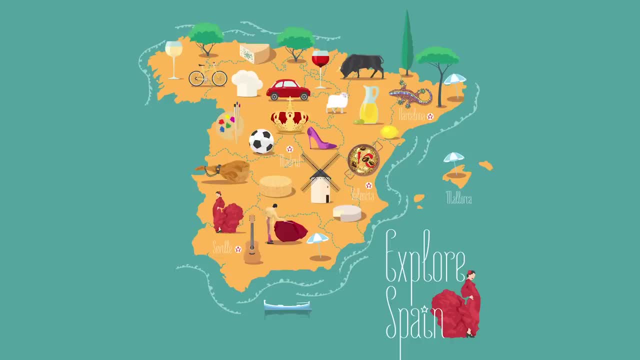 The Chinese culture has six different languages, but Mandarin is the most widely spoken and you can thank Chinese culture for martial arts like kung fu, silk, the animals of the Zodiac, philosophers like Confucius and other things that have spread around the world. Finally, let's talk about the Spanish culture. Their food often includes a variety of food, such as eggs, meat, fish, water and meat. The Chinese Chinese culture is all about their culture and food In the Chinese culture. the Chinese culture is the most popular and it is often used as a way to 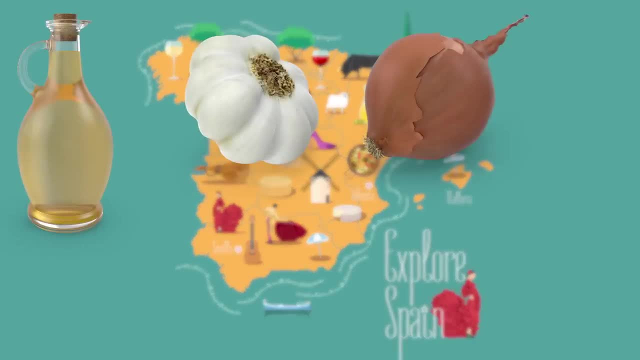 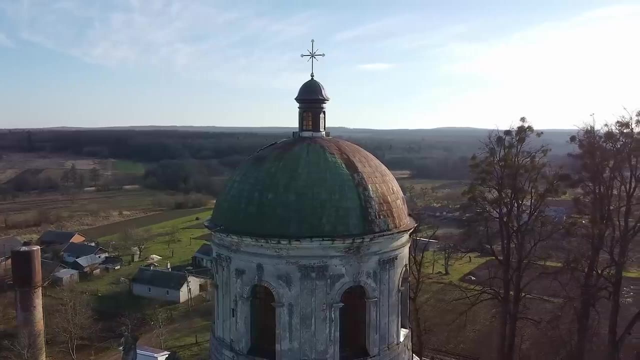 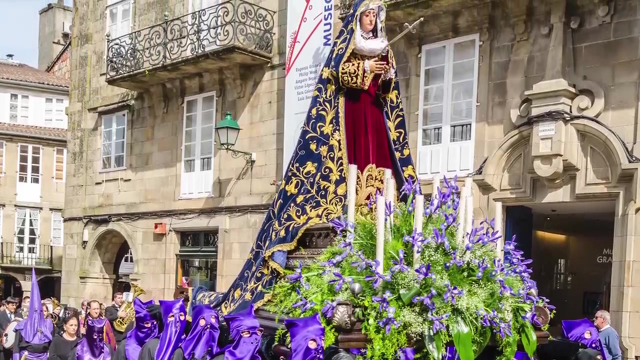 olive oil, garlic and onions. They usually serve wine during dinner and bread with nearly every meal. Fruit is the main dessert. About 80% of the Spanish are Roman Catholic, which is a form of Christianity. An important week in the Spanish culture is Holy Week, which comes before Easter. 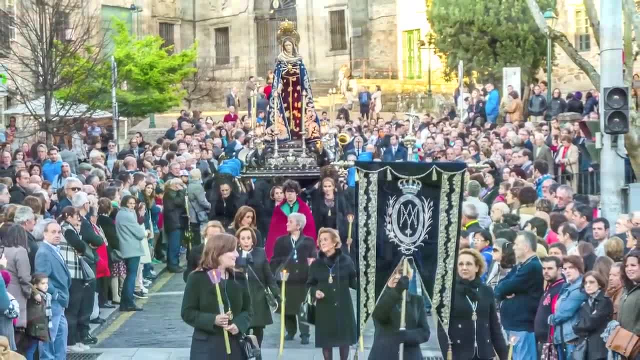 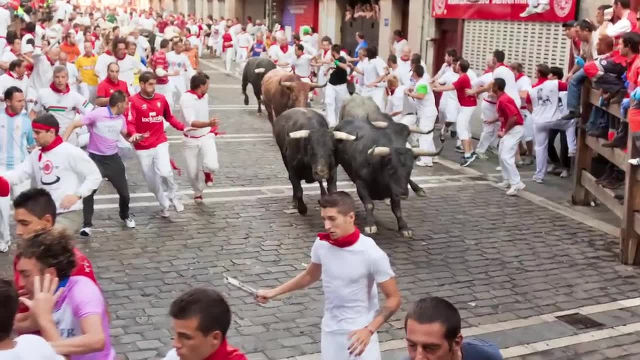 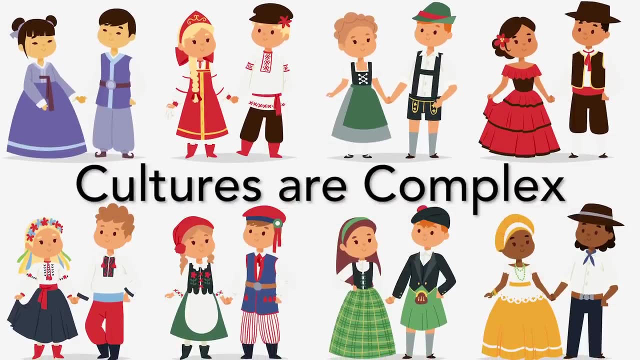 in which there are large parades and religious events. Spanish culture has colorful architecture, grand churches and even the running of the bulls. Now that you know some of the elements of various cultures, it's important to note that cultures are complex and that no single aspect of a culture defines it. They can be so local that different. 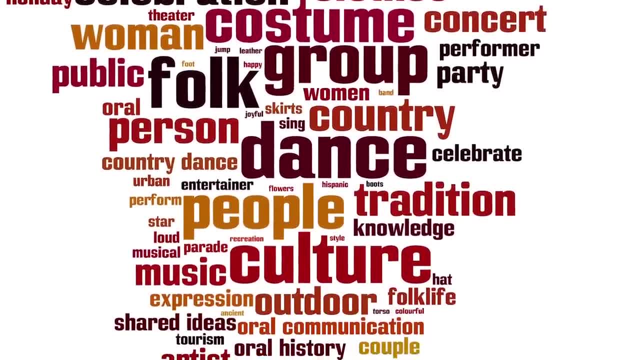 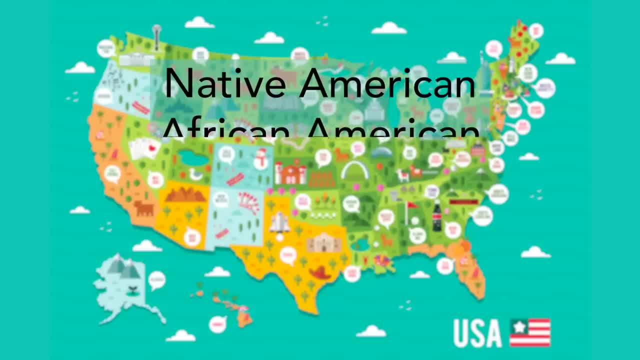 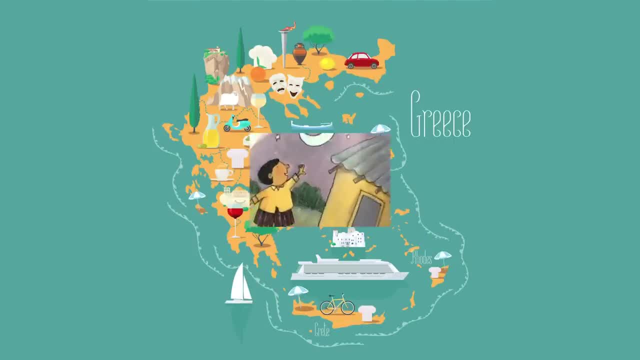 people in different parts of a country can have vastly different things that they cherish and celebrate. In America you have Native American culture, African American culture, Cato and many more- Asian Creole and others. In Greece, a child throws a lost tooth onto a roof for good luck. 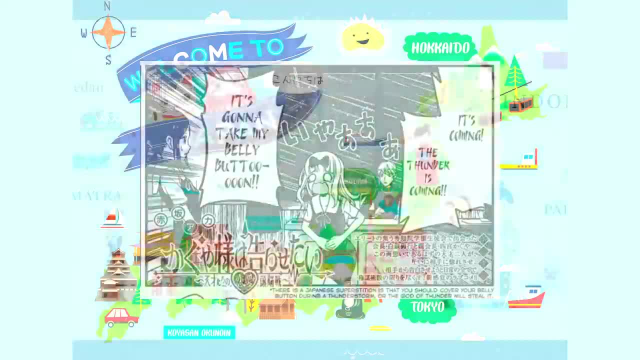 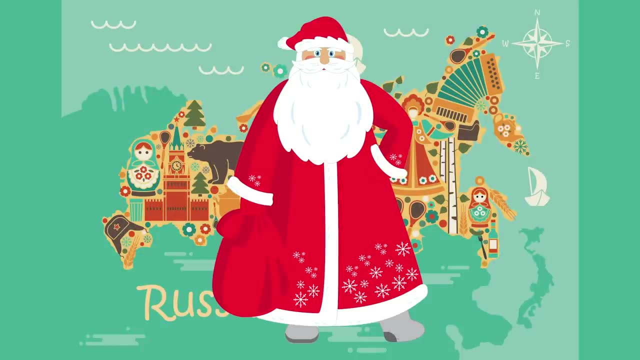 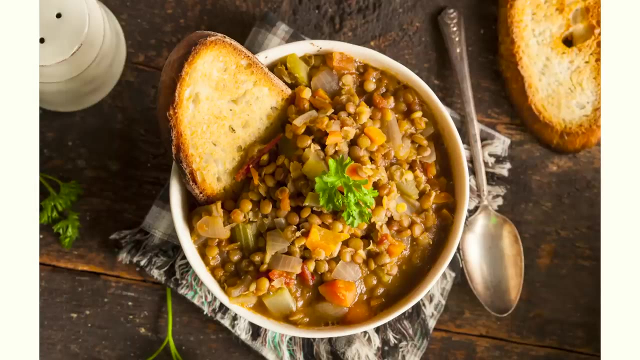 Japanese children cover their belly buttons when they hear thunder. In Indonesia, people point with their thumbs. In Russia, Father Frost brings children presents on New Year's Day. In the Brazilian culture, New Year's Day is usually celebrated with a bowl of lentil soup. Now that's.